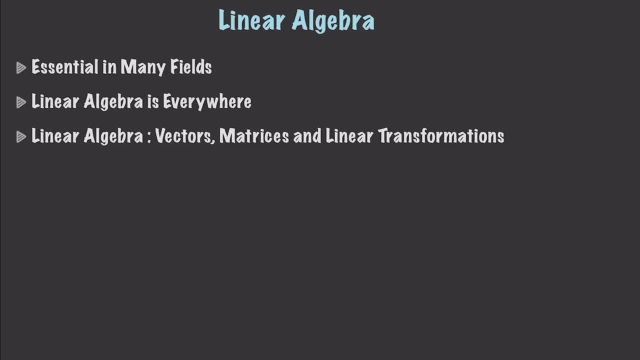 is great about it is that it allows you to model relationships between multivariable inputs and outputs, And what I'm going to do is sort of bounce around a lot in this video. One thing that I'm going to do is I'm going to talk about some symbols. So if you ever see a symbol like this, it's an R. 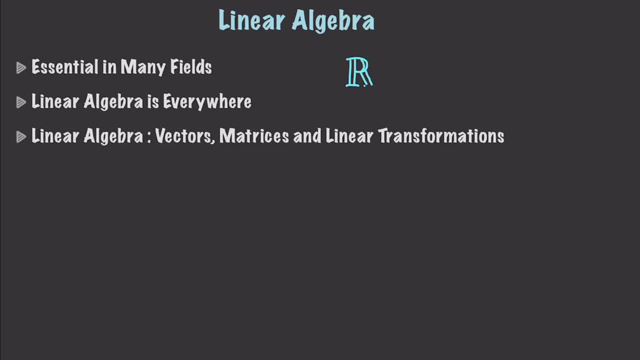 what it represents are all real numbers And if you ever see something that looks like this, this symbol is saying that it represents an array of real numbers, with three rows- The rows always come first- And two columns. This symbol down here with its V, with a little arrow. 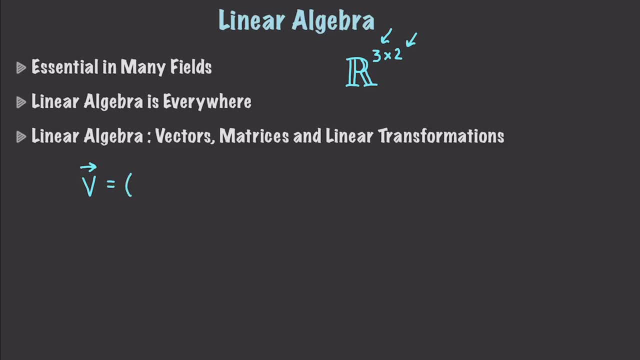 over top of it is going to represent, in this situation, a two-dimensional vector, And if we should come in and throw in another value, this would represent a three-dimensional vector, And a vector is going to represent a three-dimensional vector, And if you ever see a symbol like this, 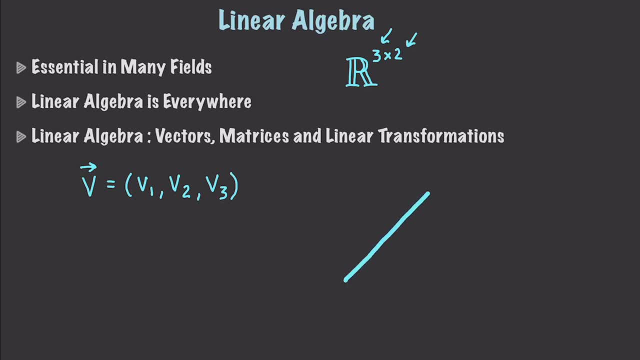 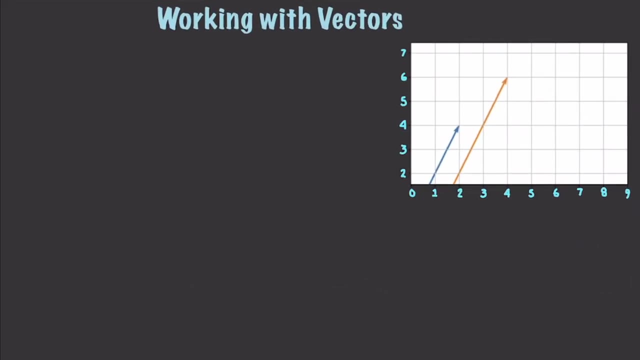 is going to have a direction as well as a magnitude, And now what I want to do is jump in and talk about different ways that we can manipulate vectors. Now, the very first thing I want to talk about is scaling a vector. Scaling a vector. 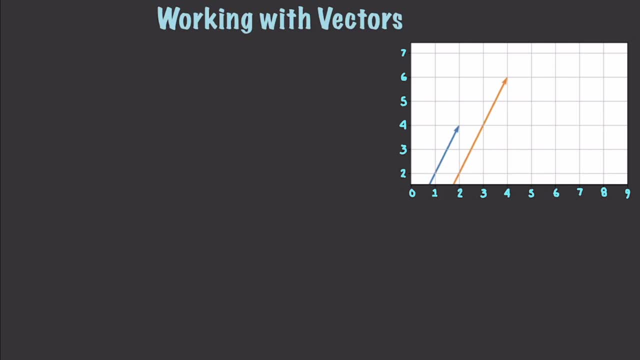 involves multiplying all values in a vector by a scalar, which is just a value with magnitude but not a direction. So let's say we have a vector and we want to scale it by 2. We are essentially just multiplying it And you can see an 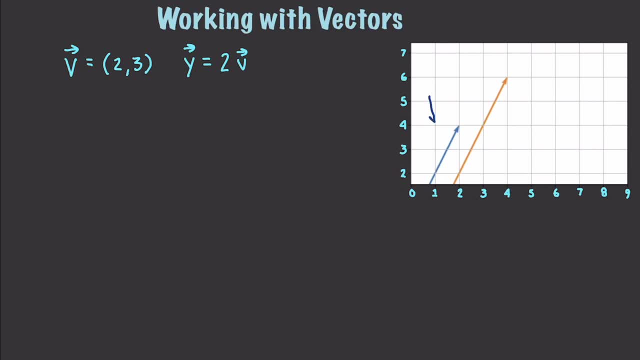 example over here in our graph, of exactly what would happen. This is the original vector and this is the scaled vector. If we wanted to add vectors, let's go and let's just keep the 2, 3 here and let's add a new vector, y, Simply adding. 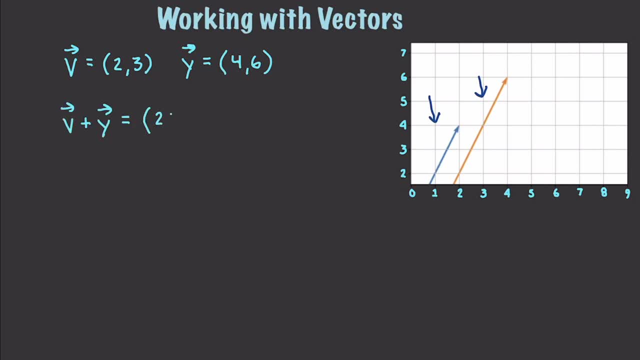 these together means that we will take the 2 and add it to the 4, and the 3 and add it to the 6, giving us a final answer of 6 and 9.. Subtracting them works probably the way that you would guess that it would work In this situation. we. 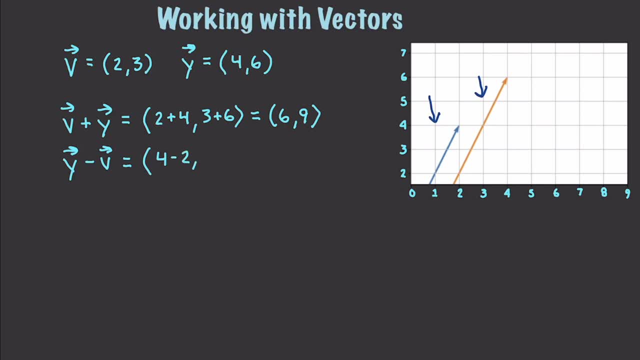 would just take the 4, subtract the 2 from it, take the 6 and subtract the 3 from it to get a final answer of 2 and 3.. Now, dot product is going to take two vectors and return a scalar. Remember, scalar has magnitude, no direction, And you're going to 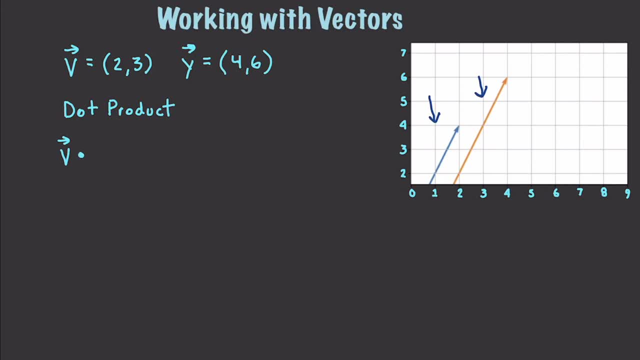 designate that this is a dot product by putting a dot inside of here like that. And how you figure this out is you would take Vx times Yx plus Vy times Yy, And this, of course, is going to work out to being 2 times 4 plus 3 times 6.. And this would continue on if you had a three. 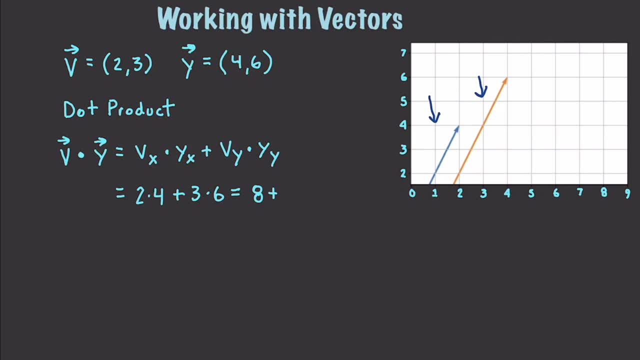 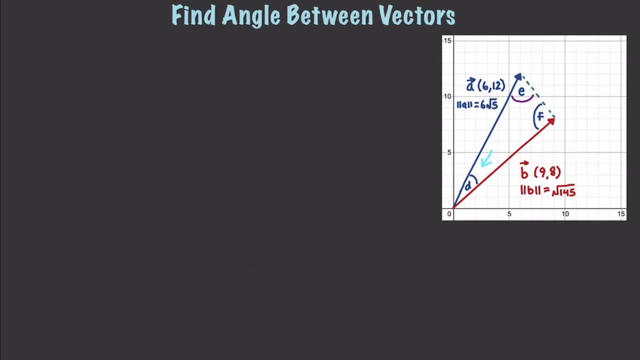 dimensional vector And you'd get a final value of 8 plus 18, which is equal to 26.. Now, one thing that is very useful in regards to the dot product is it's going to allow us to find the angle between vectors. So let's say we want to find this angle right down. 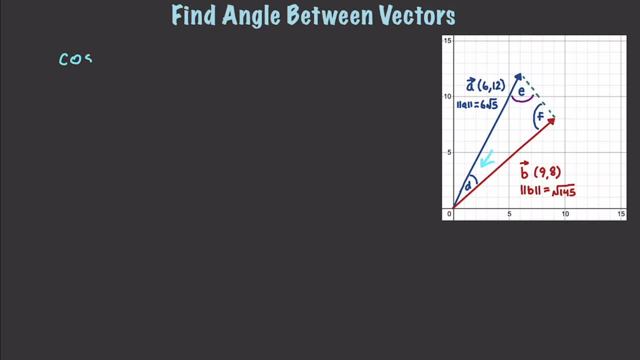 here D. Well, what we would do is we would say: cosine of D is equal to the dot product of A and B, And you can see the values of A right there and B right there. And you can see the values of A right there and B right there. And you can see the values of A right. 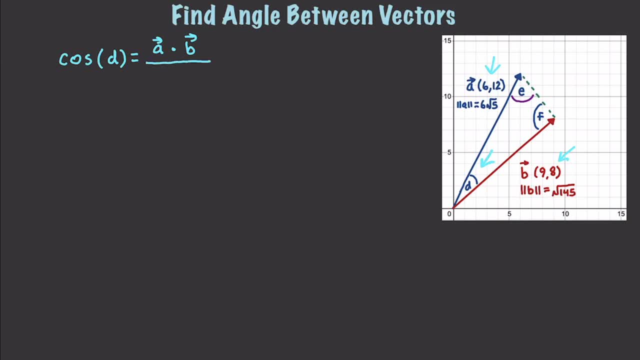 there, Divided by the magnitude of A times the magnitude of B. Well, how do you calculate the magnitude? Well, I'm going to show you how to calculate the magnitude of A. It is going to be equal to the square root of A1 squared plus A2 squared, And this is going 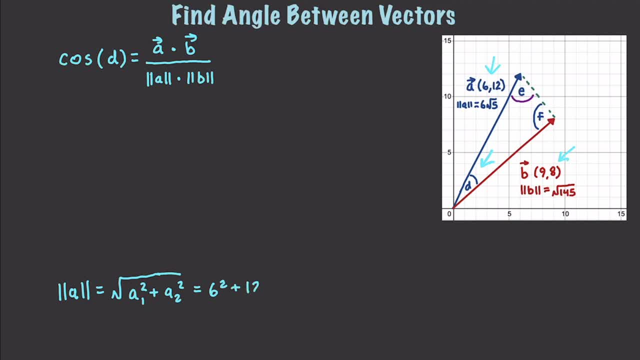 to work out to be 6 squared plus 12 squared, Square root of that. And then, if we were to simplify this, I'm going to take you through the whole process. This is going to be 36 plus 144, which is equal to square root of 180, which we can simplify down into the square. 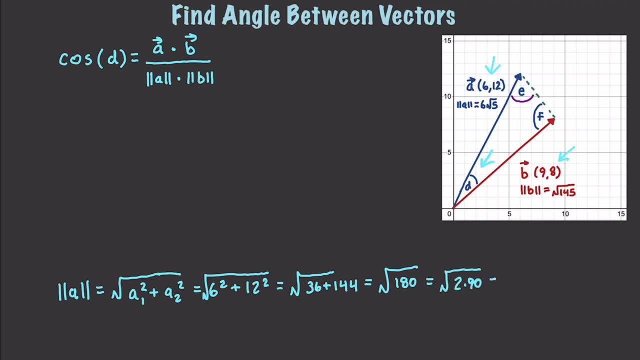 root of 2 times 90.. I'm going to ha segu all the way down into square root of 24 to get us down till the вас окой. do a simple��� speed in here. The next thing you need to do is charities of help is all we need to do is to root round. 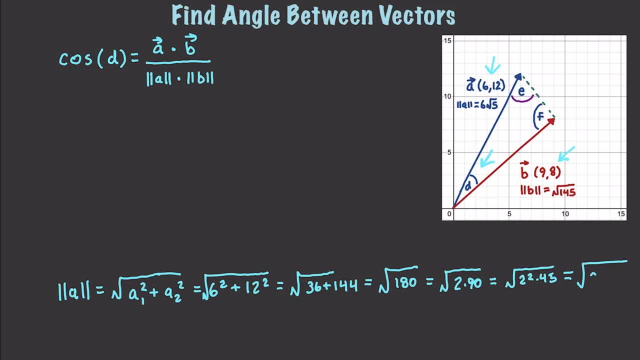 across this circle. So number three, number three times x5.. I'm going to use this simple function over here, just here, which is going to be the square root. I am just going to do this over here. So remember, this will be the square root of x1, squared Here you. 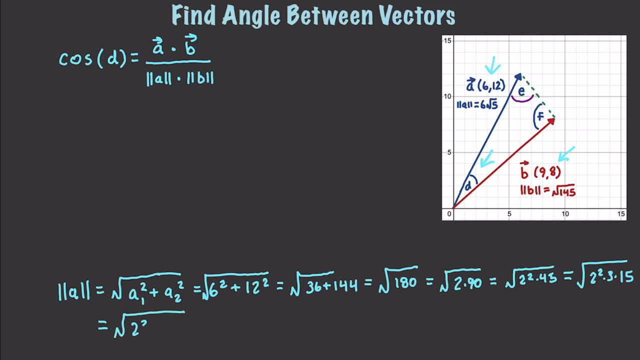 are going to have the sites of x1 squared, and I know that it is the sameここ. this is the same, plus the square root of x1 squared. here we are going to take a integral slide over to x1 squared times xmin than 320.. Now switch the two. So here we have 25 squared times. 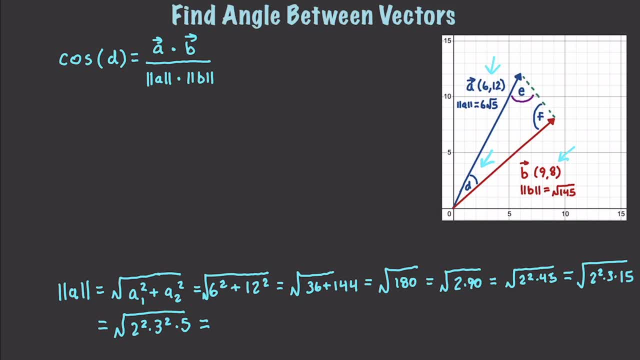 140.. Okay, all right times five. and then we can finally simplify this by getting rid of this two and this squared part. multiply the two times the three, which is going to equal six times the square root of five. so that is the magnitude of a. so you can go and practice and figure out the magnitude of b. but what i'm 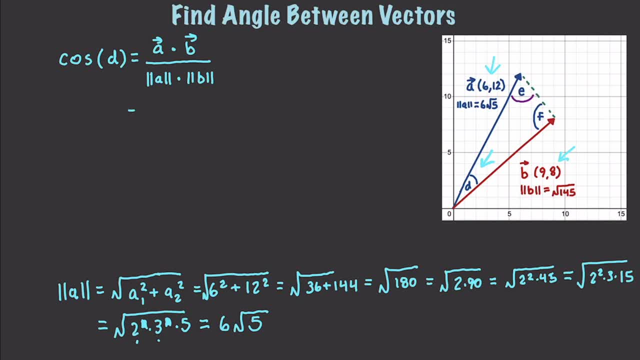 going to do is just solve this. okay, so we're going to get our dot product here. so this is going to end up being six times nine plus 12 times eight over the magnitude of a, which, as i showed you, is six times the square root of five times, and the magnitude of b is the square root of 145. 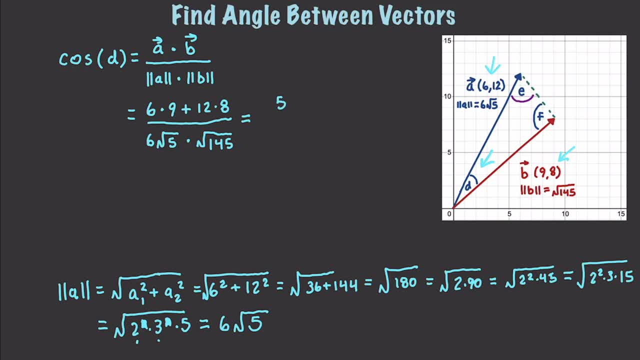 this is going to further simplify down to be 54 plus 96 and we work these out. this will be 13.416 times 12.042, which is going to be equal to 150 over 161.55, which is going to be equal to 0.9285. then what we can do is we can take the arc cosine of 0.9285. 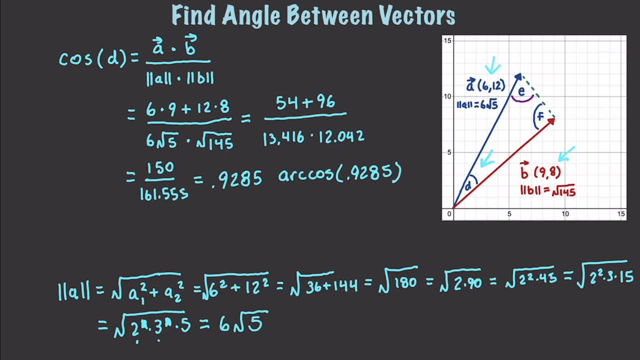 and that is going to give us our final radian value for our angle d of 0.3804. if we multiply that, then times 180, divided by pi or 57.296, which is that value, that is going to tell us that the angle for d is 79 or 21.79 degrees. all right, so learned a whole bunch of things in that one little. 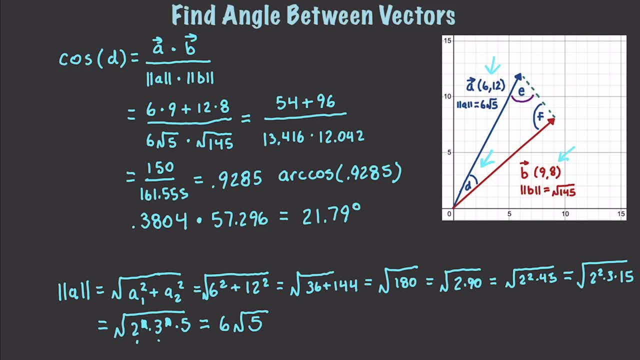 example and some points that are important to know. as if, because I'm goes 0.6, well 10owers is equal to 1, then what that tells you is that the vector a and b or pointing in the same direction. if, however, co's sign of 90 degrees is equal to 0, that means that those electors or 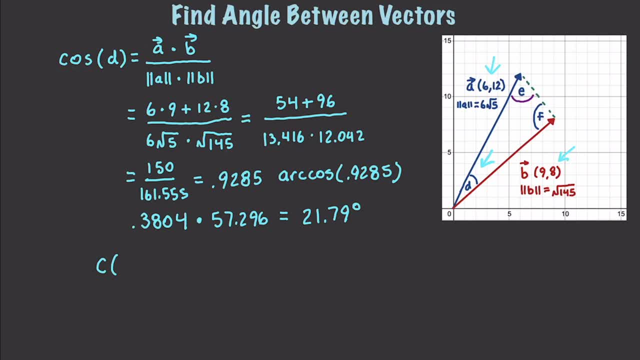 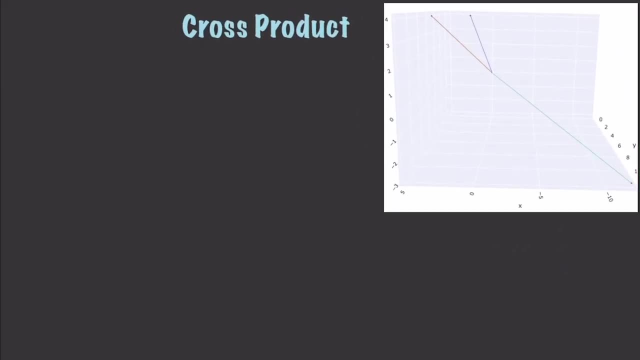 pointing in opposite directions and in a situation in which we had cosine all of 10 and 80 degrees, equal to negative 1, that means that those vectors are perpendicular And that moves us on to the cross product. Basically, what it's going to do is it's going to take two vectors and then it's going to 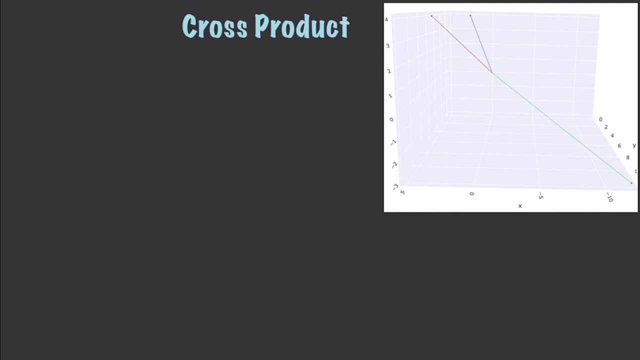 return a vector that is at right angles to both. And something else that's important to remember is that if the cross product is 0, that means that the vectors are going to be pointing in the same or opposite direction And the cross product is going to be at a maximum length when vectors A and B in this 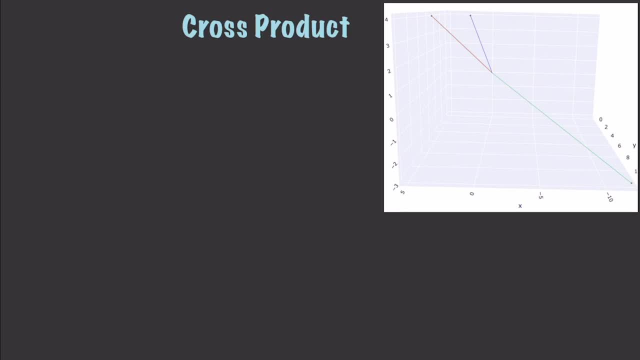 situation are at right angles. So if you want to calculate the resulting vector using our two provided vectors, which is 2,, 3, and 4.. And B being equal to 2,, 5,, 6, and 4.. 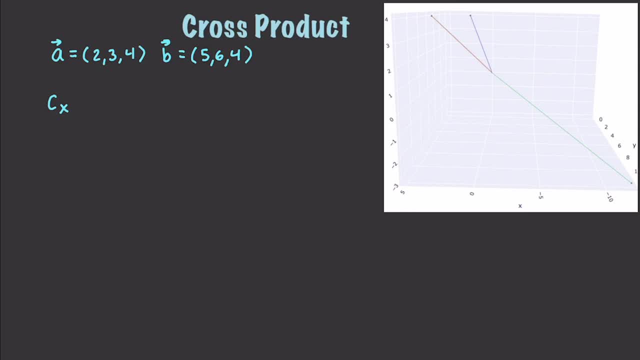 How you would do that is, the resulting vector CX is going to be equal to AY, BZ minus AZBY, and CY's value C, representing the resulting vector from this use of cross product, is going to be AZBX minus CY. Okay, 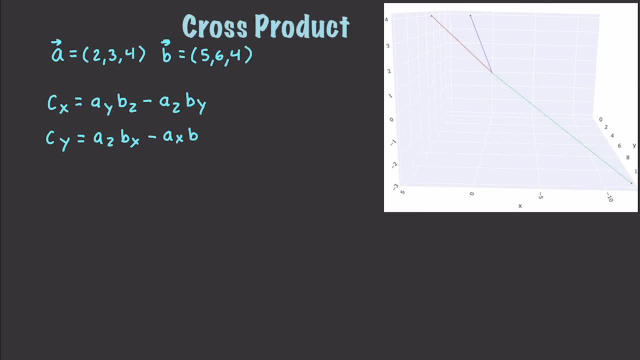 So that's going to be 3 times 4 minus AXBZ, And CZ is going to be equal to AXBY minus AYBX, And if we want to go and solve this, the resulting vector C is going to be 3 times. 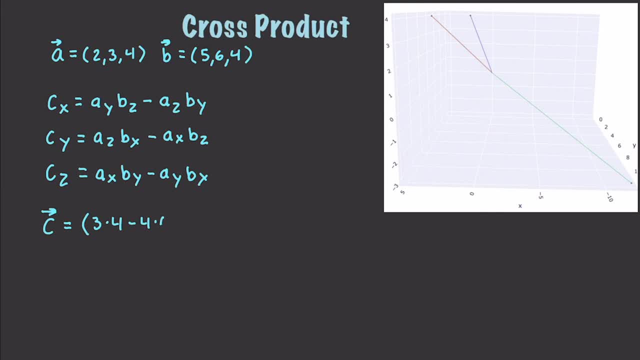 4 minus 4 times 6.. And 4 times 5 minus 2 times 4.. And 2 times 6 minus 3 times 5,, which is going to give us a final vector of negative 12, 12, and negative 3.. 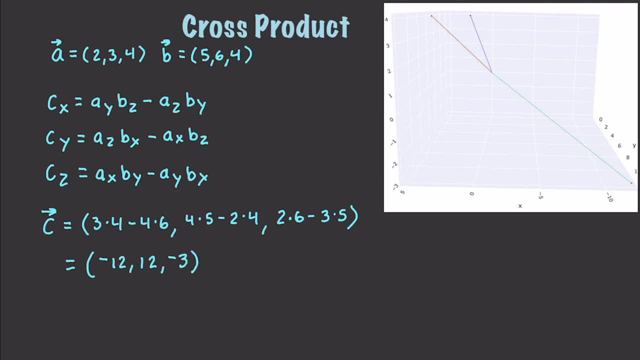 And you can see that plot right there on the right side of your screen. And this right here, this blue line, is going to represent vector A, This one right here is going to represent vector B And this one right here sticking out really far, is vector. 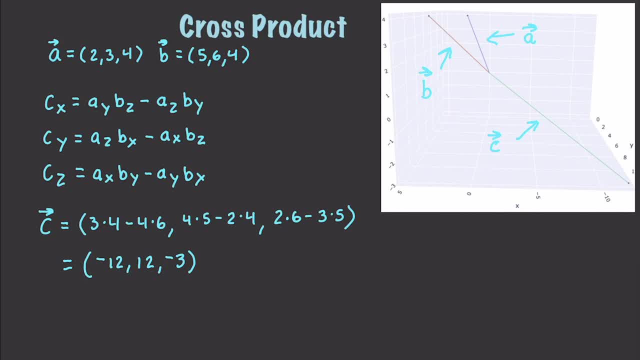 C. Something else that is important before I move on to matrices, is that a unit vector is going to have a magnitude of 1.. Okay, So let's say we have a vector to demonstrate this and I'm going to leave it be A in this. 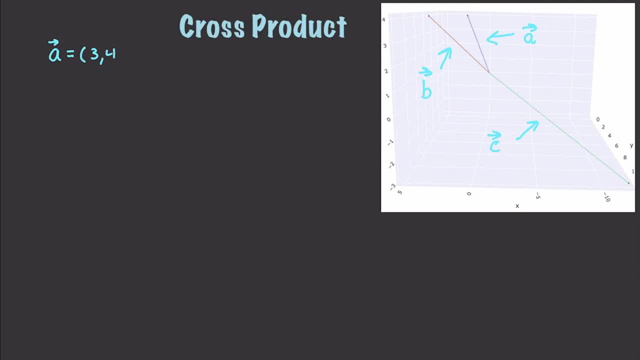 situation, but I'm going to give it different values, so it's going to be 3 and 4 in this situation. Well, if I want to go and get the magnitude of this, this is going to work out to be 3 squared plus 4 squared, just as I had shown you a couple of seconds ago, which works out. 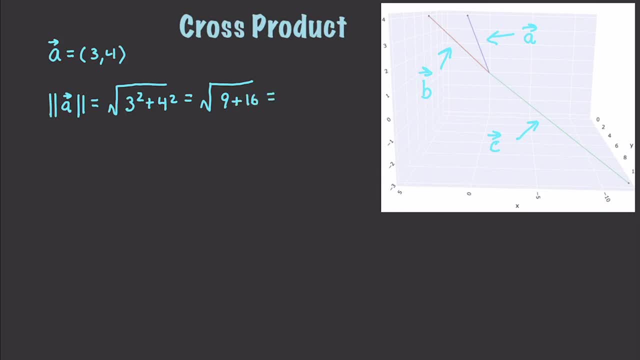 to be 9 plus 16,, which is equal to the square root of 25,, which, of course, is equal to 5.. Alright, to find the unit vector, what you need to do is to divide both of these parts of our vector by the magnitude. 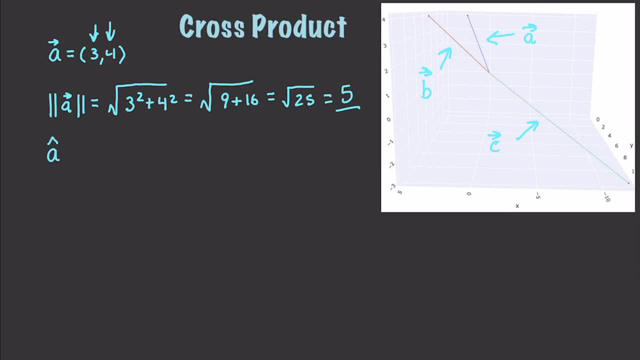 And you're going to represent the unit vector by changing it to A hat. So this is going to be equal to 9.. 3 over 5 and 4 over 5.. But how do we verify that this is indeed a unit vector? 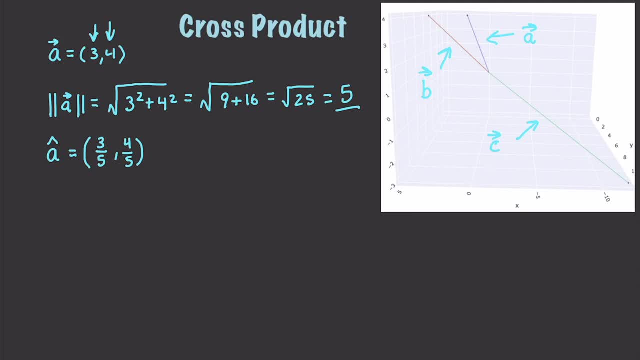 Well, if we go and get the magnitude of it, we're going to find out that it has a value of 1.. And so let's verify. So let's say we have 3 over 5, and this is going to be squared plus 4 over 5, also squared. 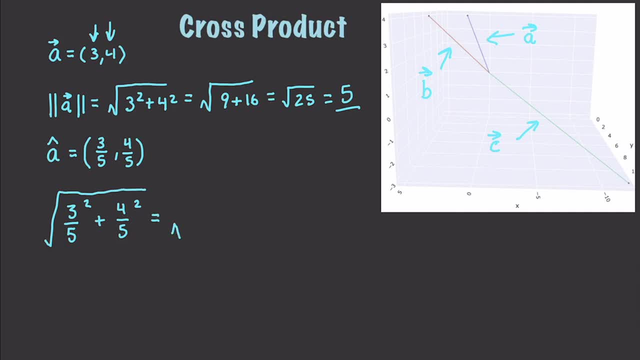 root, of course, And this is going to work out to being 9 over 25 plus 16 over 25, which is equal to the square root of 25 over 25, which I'm sure you know is equal to 1.. 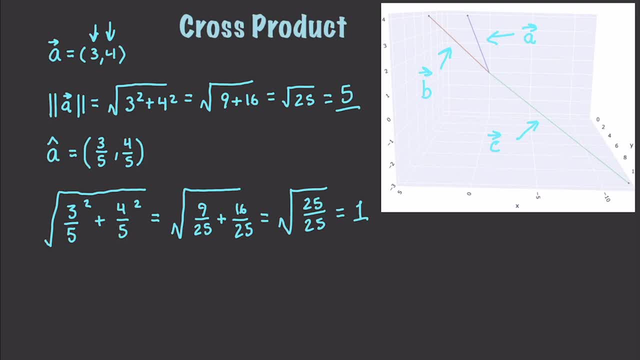 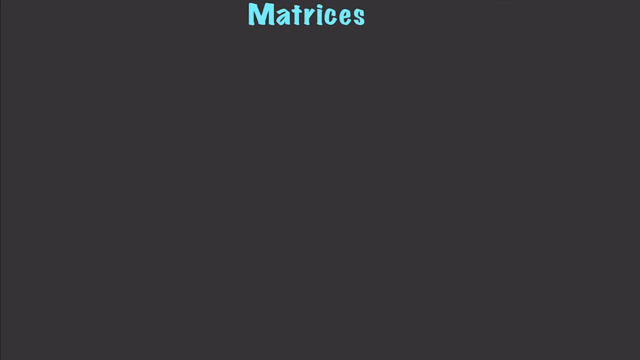 Alright. so we did a whole bunch of different things here with vectors, and now I want to give just a brief overview of matrices so that you can see how important they are. OK, so a matrix is just an array of numbers, Or it could just be an array of number, alright, 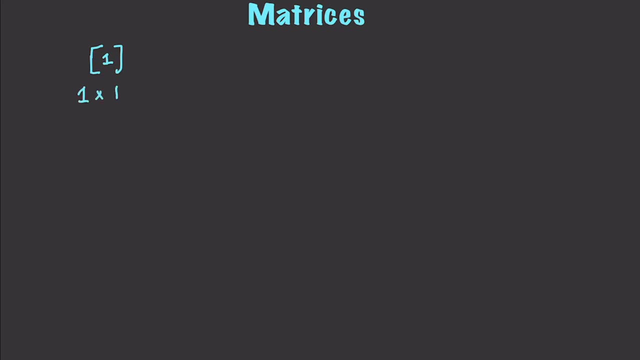 And this is what we would call a 1 by 1 array, And what these matrices are going to allow us to do is to organize data in a way that makes it easy to work with that data, And previously I showed how to find values for X and Y using matrices, and I'm going 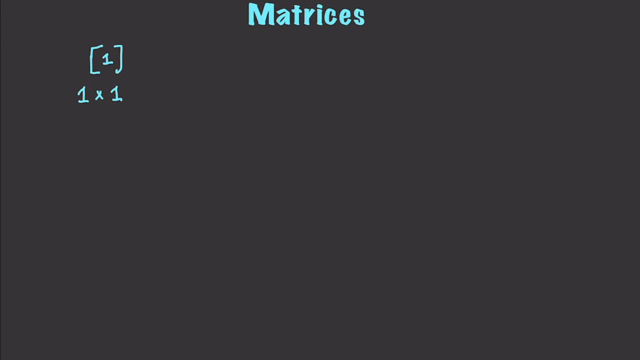 to kind of review that right now. But if you think about it whenever we are in my Algebra tutorial or using basic algebra techniques, it's not that hard to go and solve maybe two or three equations. However, it is very hard to say solve 100 equations or 1,000 equations. 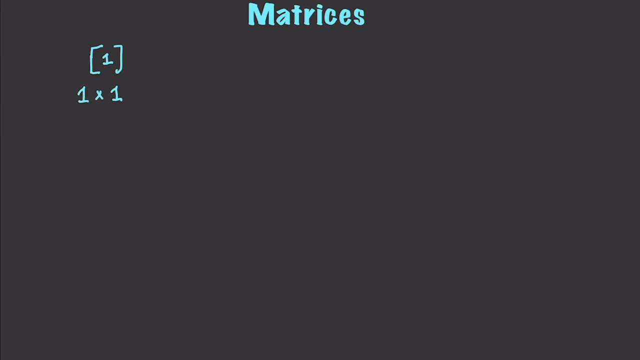 And that is one of the benefits of linear algebra in general And working with matrices. So I showed you a 1 by 1 matrix. Here is an example of a 2 by 2 matrix. And again we define our rows first, then our columns. 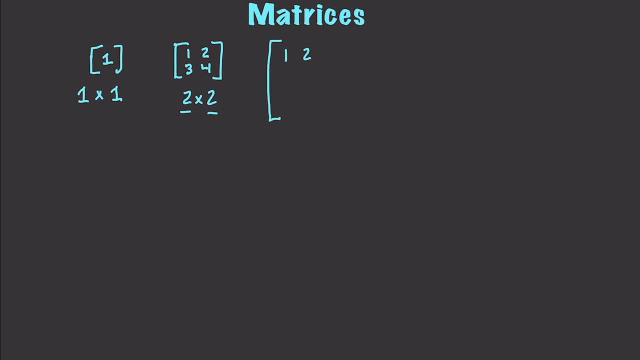 And then this would be an example, say, of a 3 by 2 matrix. alright, So this is 3 by 2.. OK, Again rows, then columns. Now, a linear system is a system of linear equations with unknown variables that are: 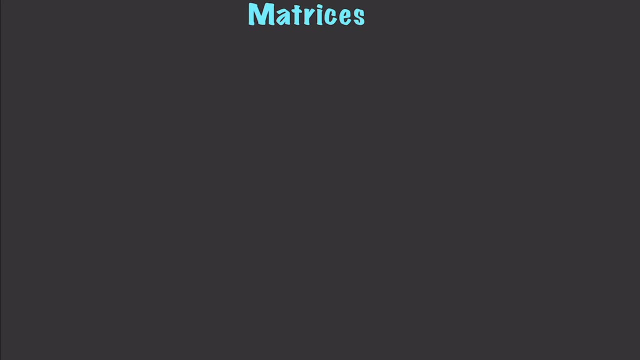 linear meaning. at most they are raised to the power of 1,. OK, So you're not going to be seeing X squared and such only X. So what I want to do here is I'm just going to solve an equation using substitution as: 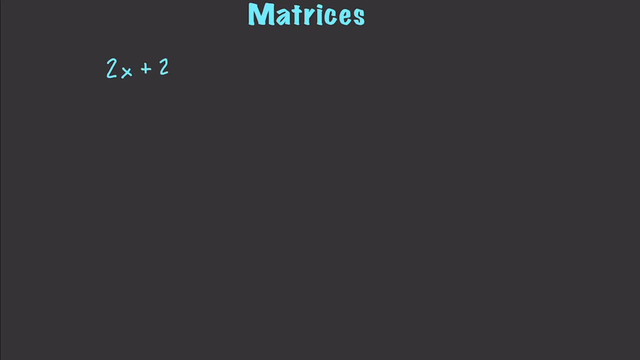 you may be aware of, And then I'll compare it to solving it using matrices So that you can see the difference. So let's say we have 2X plus 2Y is equal to 10.. And we have 3X plus 2Y equal to 12.. 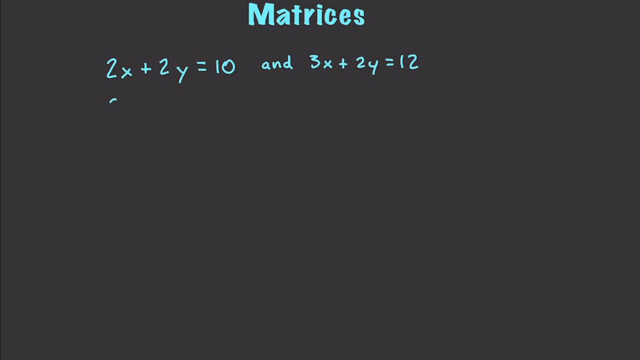 And I want to solve this using substitution. Well, what I can do is I can say: 2X is equal to 10 minus 2Y. Of course, we move this to the right side by subtracting it, And then what I'm going to do is I'm going to divide both of the values on the right side. 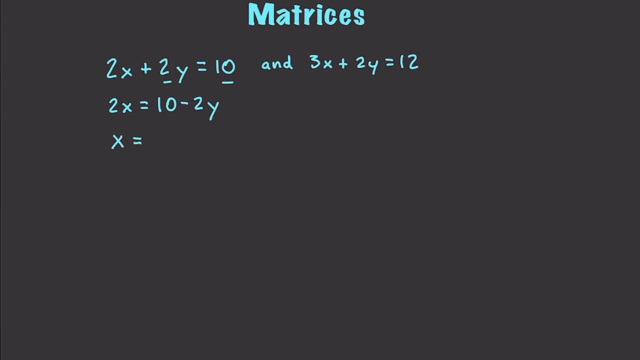 by 2, so that I can get: X is equal to 10 over 2 minus 2Y over 2.. And if I go and simplify that, that's going to give me X is equal to 5 minus Y, And then what I can do is I can transpose everywhere I have an X over in this formula. 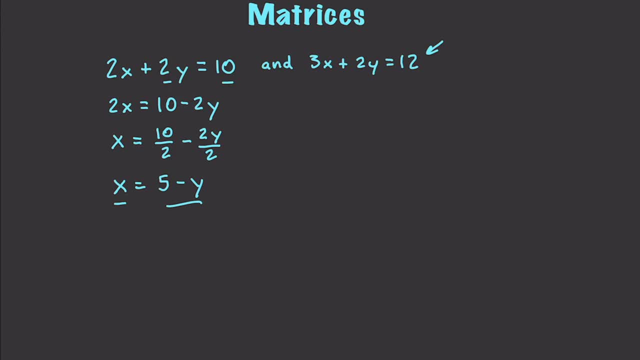 with this part And then solve to find the value of Y. So this will become 3, and then 5 minus Y plus 2Y is equal to 12.. If I multiply this through, it's going to give me 15 minus 3Y. plus 2Y is equal to 12.. 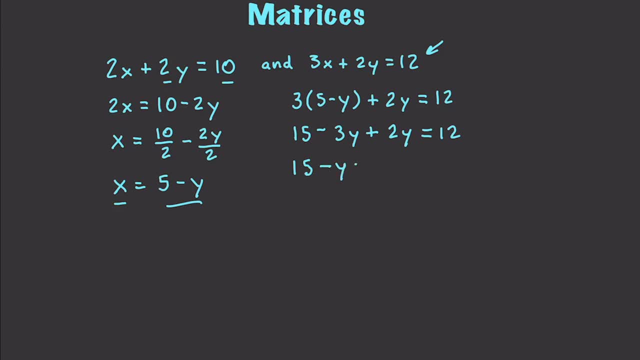 And this is going to give me 15.. 15 minus Y is equal to 12.. And of course I can then find the value of Y is equal to 3.. And then I can take this value of Y, plug it in here and find out that the value for 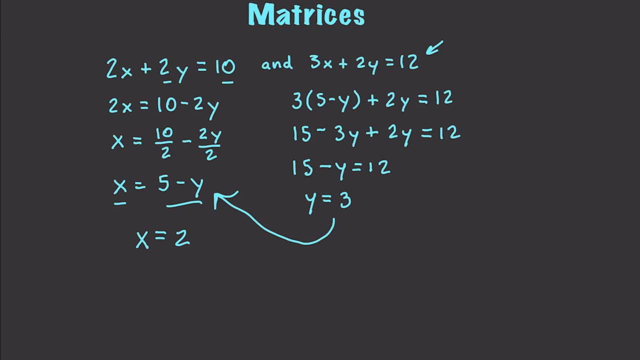 X is equal to 2, all right, And you could then verify by plugging in the value of 2 up here and the value of Y right here up here and see that this is indeed true. But I want to do the same exact thing now using matrices. 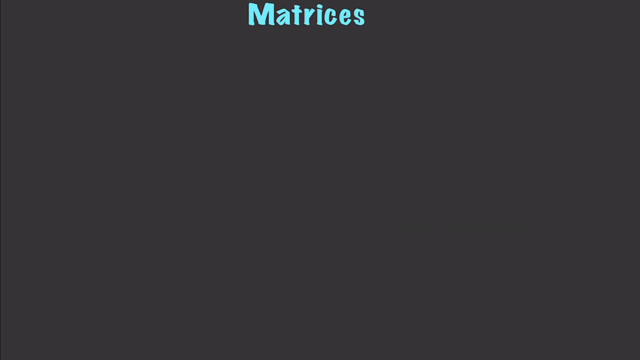 A couple of things you need to know before you proceed with doing so. Now this: well, you know what. I'm going to bring this back and I'm going to delete just this part. All right, so we have our equations here. 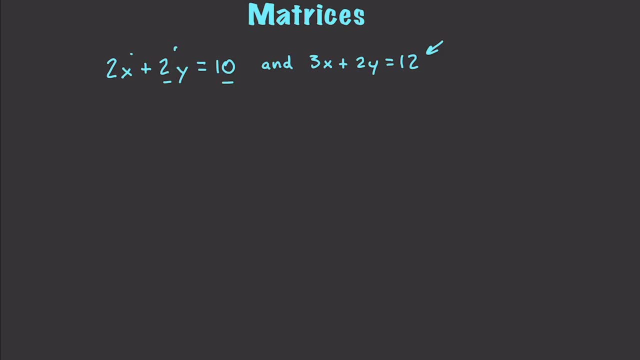 Now there are different types of matrices. If I was to go and create a matrix and I would use this coefficient and this coefficient right here, how I would line them up is I would put 2 and 2 right there. Then I could take the 3 and the 2 and put it right there. 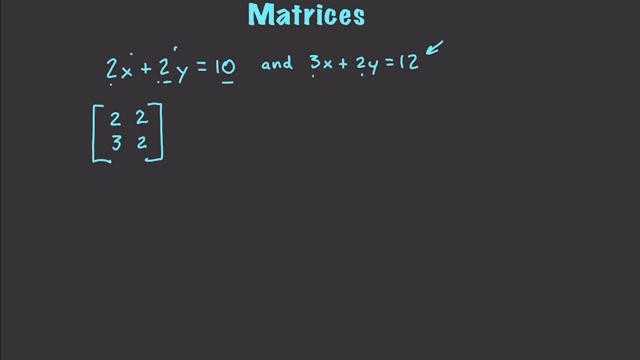 And this is what we call a coefficient matrix. Well, but I'm leaving behind my 10 and my 12 and I can't solve system equations without those, So I'm going to create 2 and 2 and 3 and 2.. 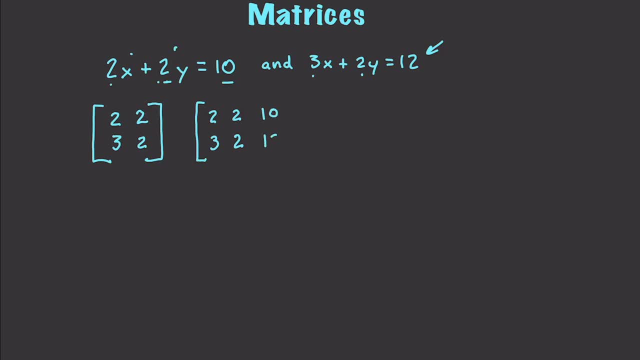 However, I'm going to put my 10 up here and my 12 right there and draw a line between it, And this is what we call an augmented matrix. all right. All right, Because we have everything here now that we can use to solve our equations. 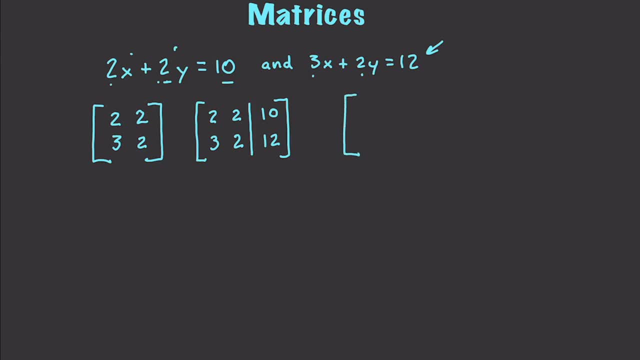 Another thing you need to know is there's something that is called an identity matrix, And all that it is is it is going to have 1s in the diagonals and 0s every place else. So that is an identity matrix, and this is an identity matrix as well. okay, 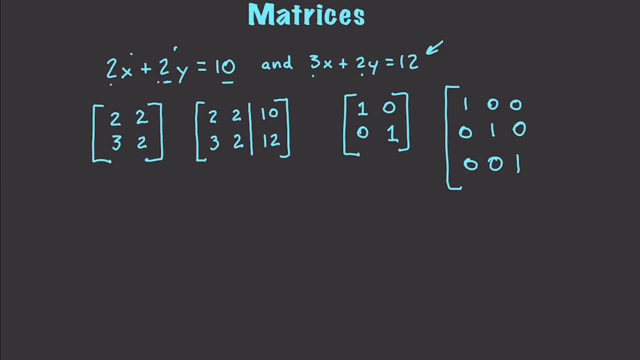 So that's the difference, or that's exactly it. So that's exactly what an identity matrix is. Now, why I told you about identity matrix is to solve system equations. you do so with matrices by converting the coefficient matrix into an identity matrix, And the values that are left on the right are your values for X and Y. 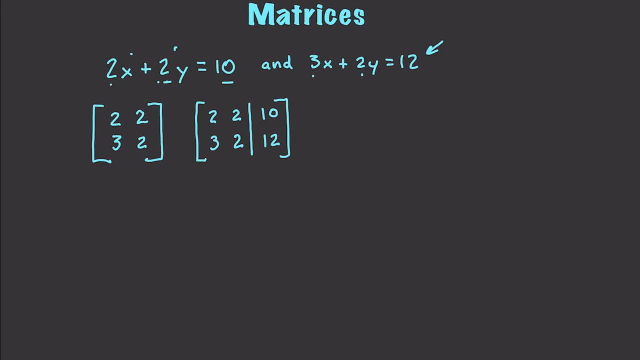 So I'm going to show you exactly how to solve this right now. So what we are simply going to do is: I have matrix, I have my matrix right here, And the very first thing you want to do whenever you are trying to solve a system equation- 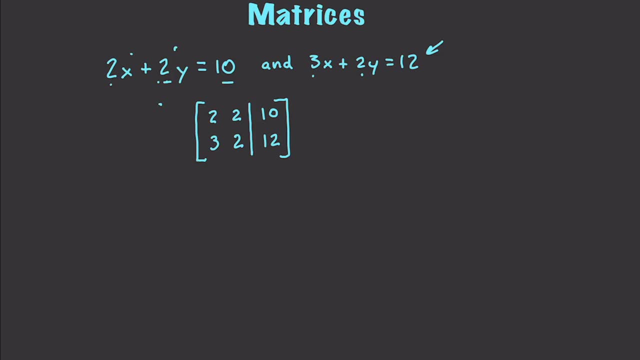 using matrices is you want to convert A11 into A1.. A11 is right here, row 1, column 1,. okay, So that's where that comes from And how you do that is by taking every value in row 1 and multiplying it by the reciprocal. 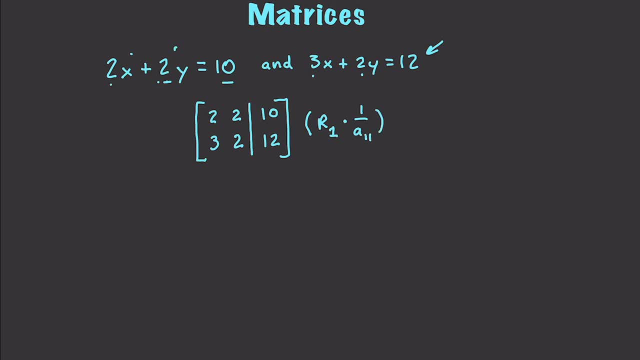 of the value of A11. Or 1 over the value of A11. Or whatever you want to think of it as, And then you're going to put that value in row 1, okay. So what's going to happen here? and I decided to move this over. we are going to go and 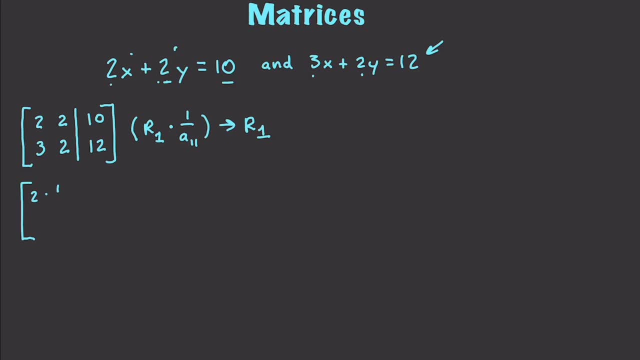 get 2, multiply it times the reciprocal of 2, which is 1 half. Do the same exact thing once again for the second row or second column, And then also do it for 10.. 10 times 1 half. We're not going to do anything on the bottom, though. 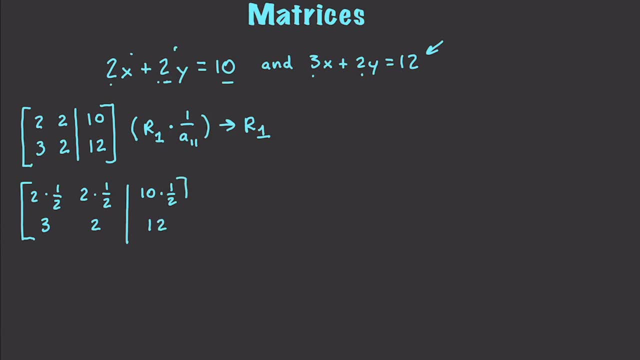 Those values are going to stay exactly as they are Now. if we do this, this is going to give us a value here with our new matrix of 1, 1, and 5, and 3,, 2, and 12.. 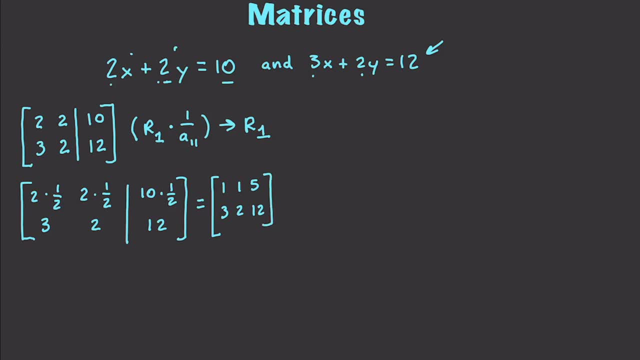 Exactly like that. Well, now what we need to do is we need to convert A21.. Or the value in the set Okay, The second row, first column, into a 0.. How do we do that? We use an equation again. 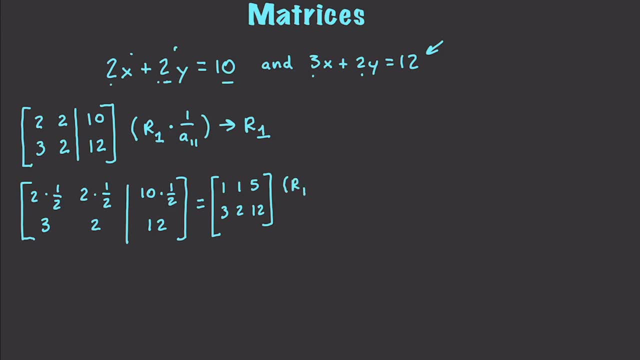 And this new equation is going to be: row 1 values times negative A21, like this plus R2, and put the result in R2.. So if we should do this, what we would end up getting is we're going to have the same. 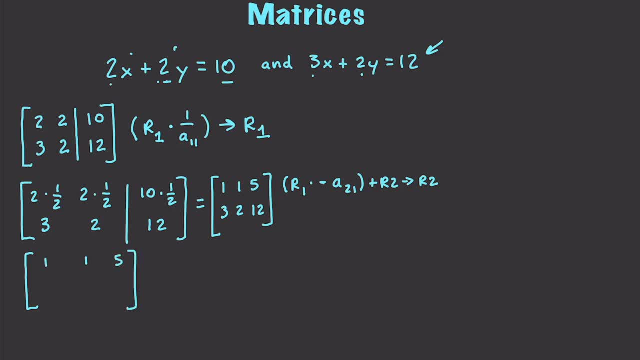 values here on the top, So 1,, 1, and 5.. Then we're going to have the value of in row 1, which is 1 times negative 3. And we're going to run out of space here. 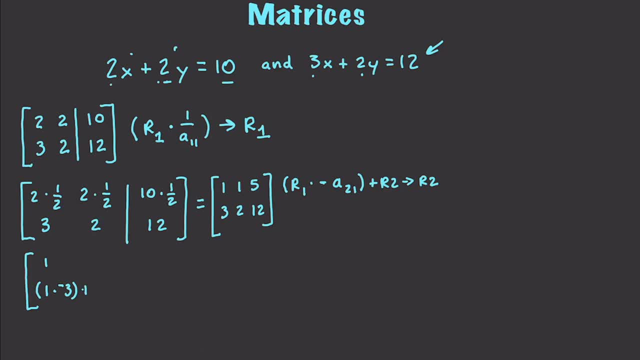 I can tell. So I'm just going to get rid of that Plus 3. And then we're going to have again row 1 times negative 3. And that plus 2. And then we're going to have 5 times negative 3.. 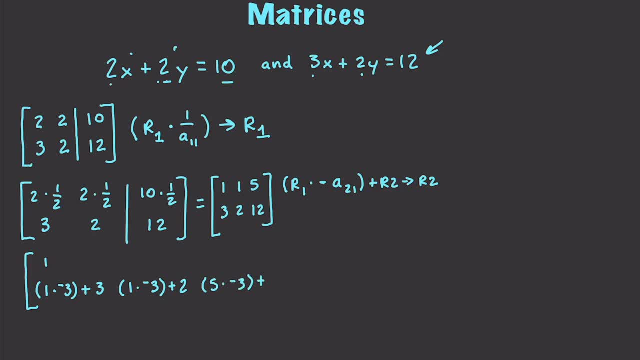 And that plus 2.. And then we're going to have 5 times negative 3. Plus 12. And if we do all of that, that is going to give us exactly what we're looking for, which is 1, and a 0, and a 1, and a negative 1, and a 5, and a 3.. 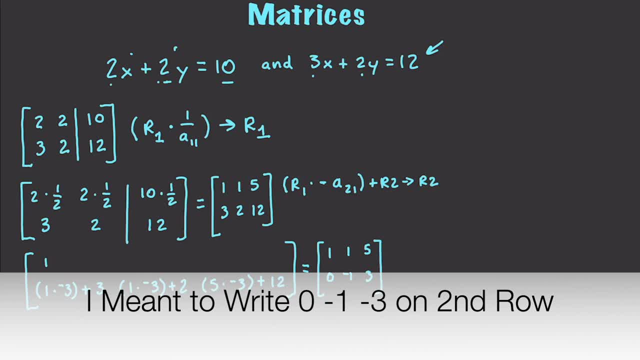 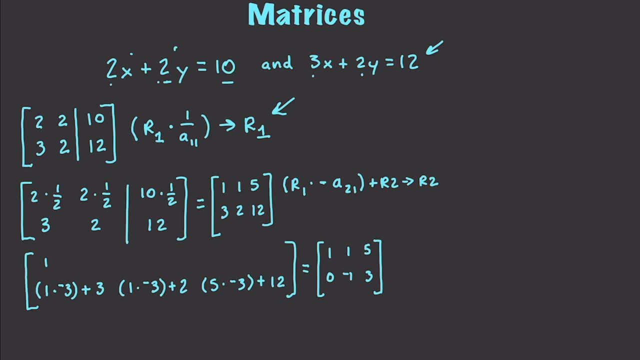 All right. So the next thing we need to do is convert A22 into A1. And the formula we're going to use is this one: right here again, except we are going to replace this- The 1s- with the 2s in this situation. 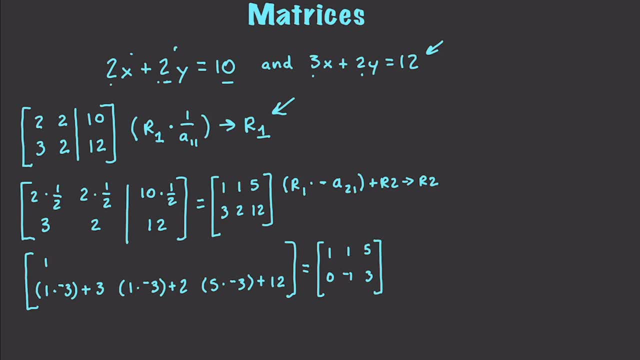 So I'm going to do that up here. So the new formula is going to be everything in row 2 divided by the value in A22 and put it inside of row 2. And if we do that, what we're going to end up having is 0 divided by negative, 1, negative. 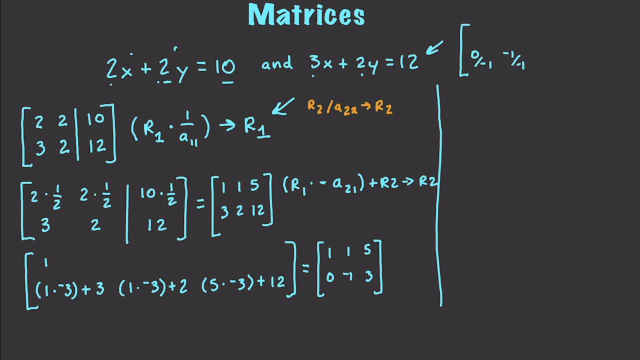 1 divided by negative 1. And negative 3 divided by negative 1.. Then we'll have a 1, and a 1, and a 5. And this is going to end up being equal to 1,, 1, and 5.. 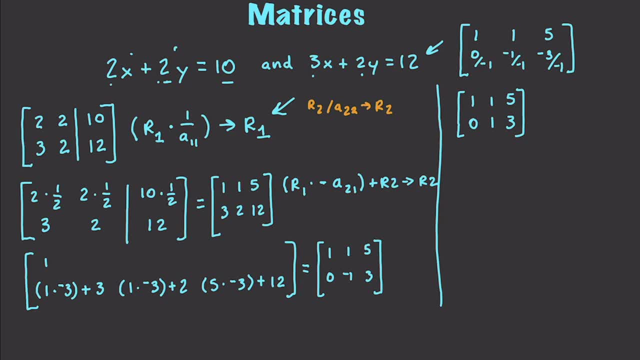 And 0,, 1, and 3.. And the only thing left to do now is to convert this up here into a 0. And how are we going to do that? We're going to use this formula, which is row 2 times negative 3.. 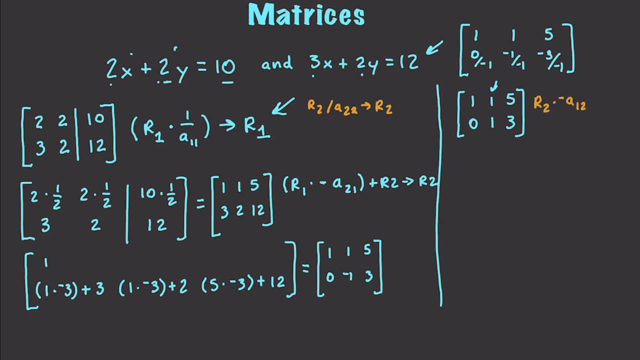 0 times negative- A12 plus R1. And put the result in R1. And if we do that, we're going to end up having 0 times negative- 1 plus 1, 0- down here And 1 times negative- 1 plus 1, 1- over here. 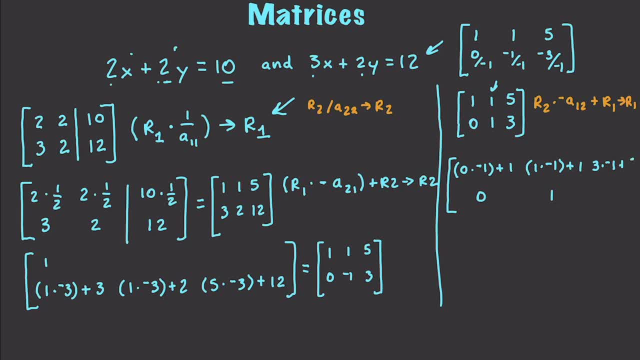 And 3 times negative: 1 plus 5.. 1 over here, 5 and 3 stays down here And that gives us a final answer for our matrix problem of 1,, 0,, 0,, 1,, 2, and 3.. 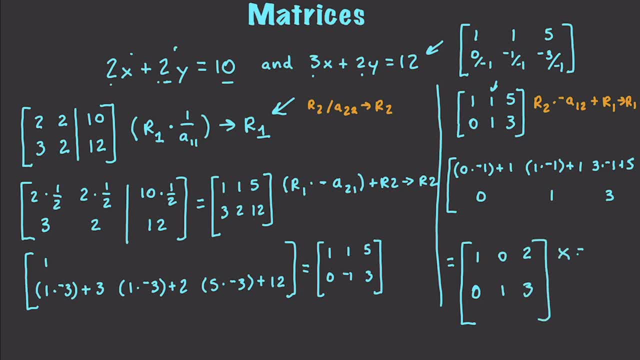 And what that tells us is that X has a value of 2 and Y has a value of 3.. And there you go, And that is how you solve systems of equations with matrices, And in upcoming videos, I'm going to show you how to do so much more. 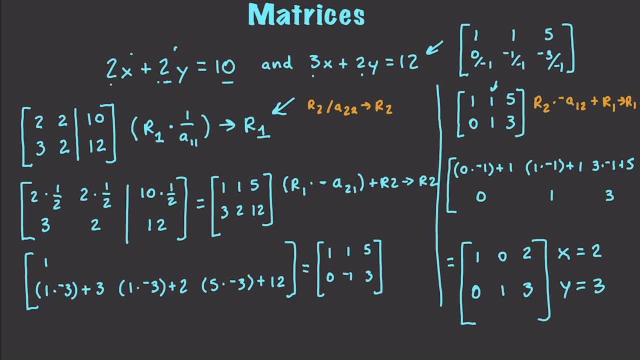 So, like always, please leave your questions and comments down below. Otherwise till next time.